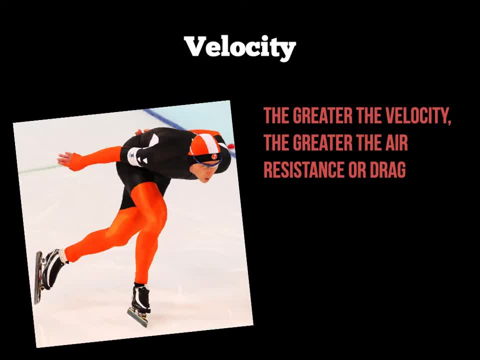 is going to be imposed on them. Think about 50 metre swimmers who are sprinters. The amount of water that comes up or the amount of drag that they create in that water is a natural reaction to how fast they're going And the reason athletes don't bother to change the 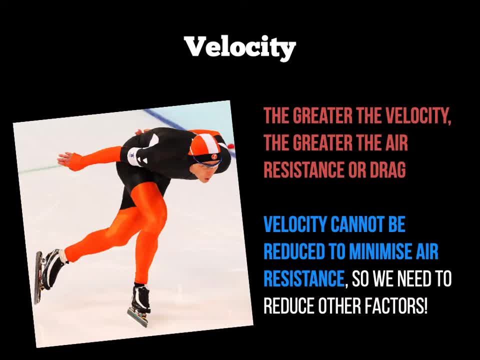 factor of velocity is because they want to go as fast as possible, And so this is a factor that's out of our control in terms of performance. We can't reduce it to minimise air resistance or drag, So we need to look at the other factors if we want to increase the speed of an object. 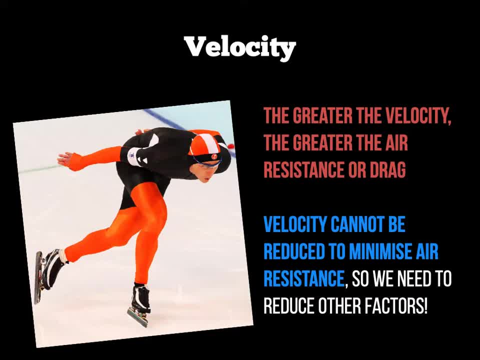 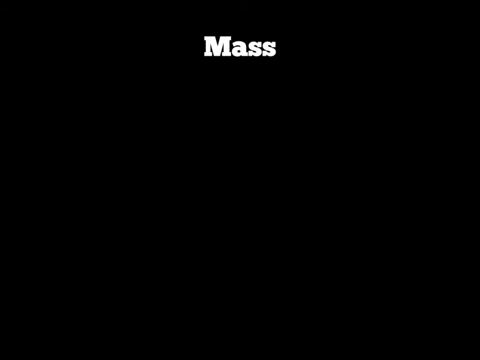 in water or in air, And so velocity is often a factor that is important, but often a factor that most athletes or top performers will not adjust. The second factor you can discuss is mass. Now, if a mass of a body becomes increased to the size, 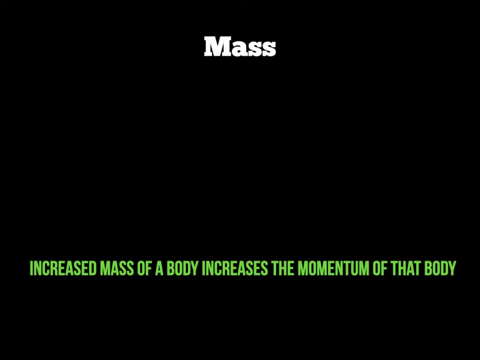 or weight of a body becomes greater. what that does is it doesn't generally factor against air resistance, but it increases the momentum of a body. So once we get that object moving because it's heavy, it's then going to accelerate fast. Think about a boulder rolling down a. 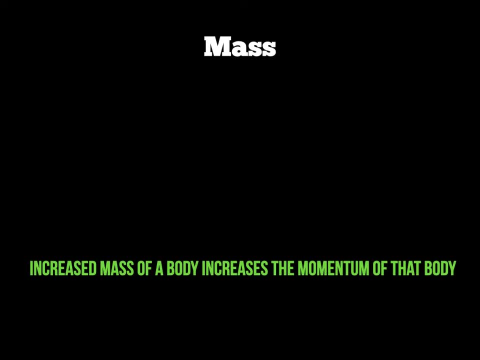 hill, We've got a heavy, massed object. It takes a while to get it going, but as it gets going, that boulder is going to accelerate rapidly, And therefore, when it accelerates, it's going to provide a lot of air resistance, And so therefore, if that body increases velocity, 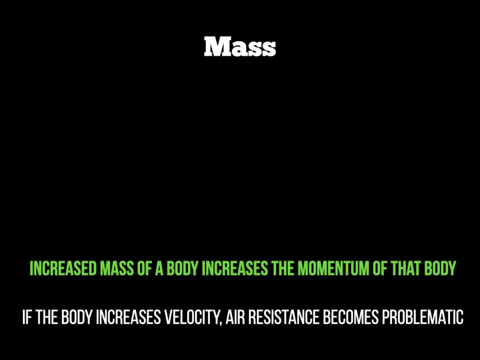 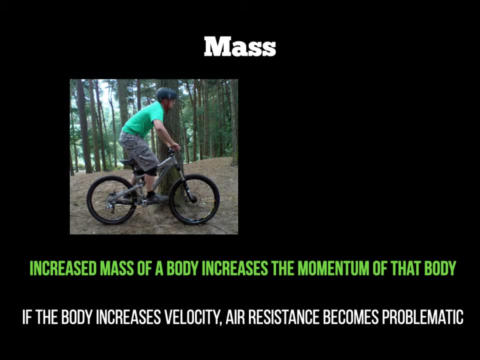 air resistance becomes much more problematic. The good example of this is something like a person on a bike, So on flat ground. if a person stood upright on flat ground, of course air resistance would meet the person themselves, because they're standing up And the bike itself weighs a certain amount. So 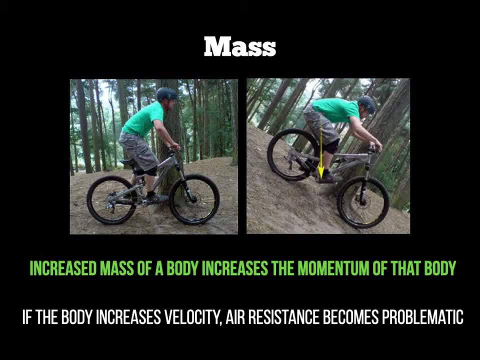 as you start to go downhill with that mass, it will take a while to generate speed, but it will start to generate quite a lot of speed And therefore the rider might need to change shape in order to manipulate the air resistance in order to go faster. So mass technically. 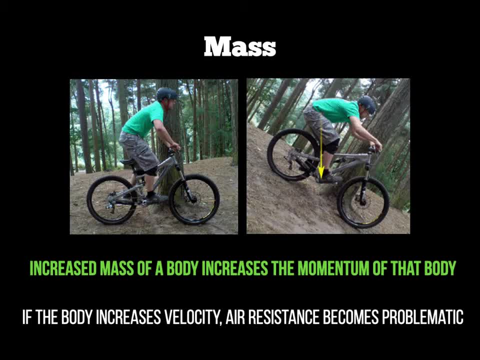 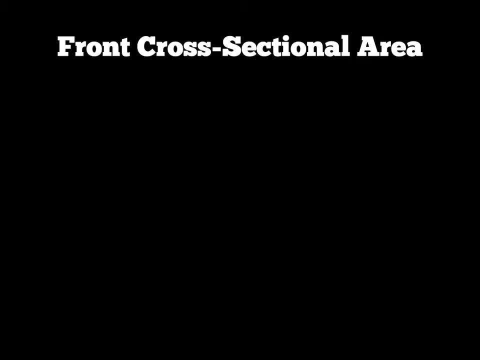 when stationary doesn't affect air resistance greatly, But once you get it going in terms of momentum, you will generate more air resistance. The third factor is front cross-sectional area. This is the area on the front of the athlete, hence the name. And the larger that area, the larger the air resistance or drag. 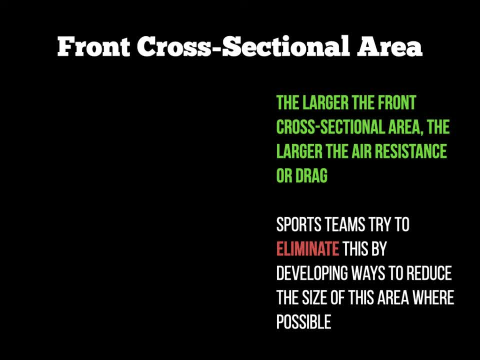 through the water, And what we know from year one work is that sports teams will try to reduce the amount of front cross-sectional area in order to get faster speeds or to accelerate athletes, because the large front cross-sectional area of an athlete will slow them down And 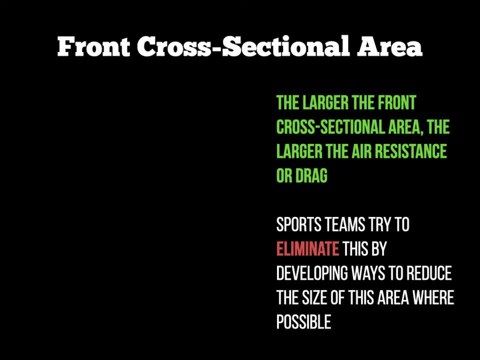 we can use things like wind tunnels, which we met in year one, to use a jet stream of coloured air to find certain positions in order to reduce air resistance and to make an athlete faster. Think about sports such as skiing- slalom skiing- The athlete will. 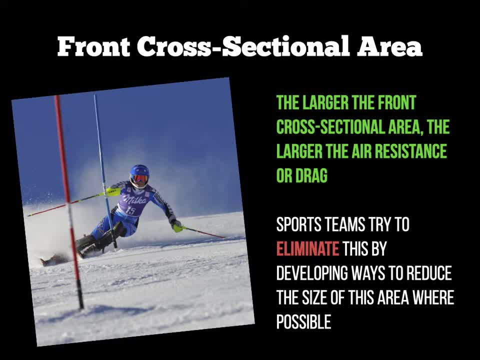 bend into a position. They'll lower the front cross-sectional area, so they bend their body forwards and they're torsional. They're also low in order to meet less air resistance and therefore to accelerate faster. The same can be said in cycling, especially when you watch track cycling, The rider will. 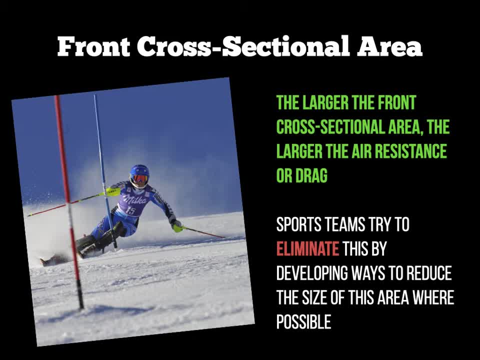 be in such a low position that the front cross-sectional area is reduced. Therefore, they can go faster In terms of cycling. if you raised your body upright while you were cycling and you were on a windy day, you would actually slow down. It'd be much harder to cycle. That's because 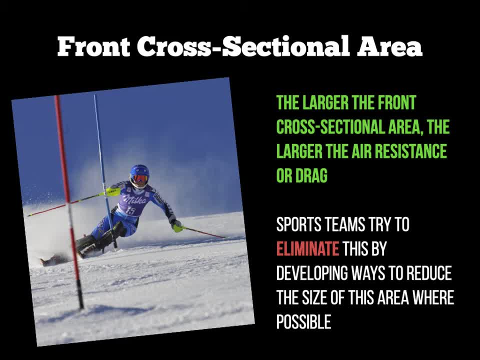 the air resistance is meeting you, And so you're going to have to slow down, And that's what we're going to talk about in the next video, Thank you. So it's that principle that athletes are trying to reduce. The same goes in the water. 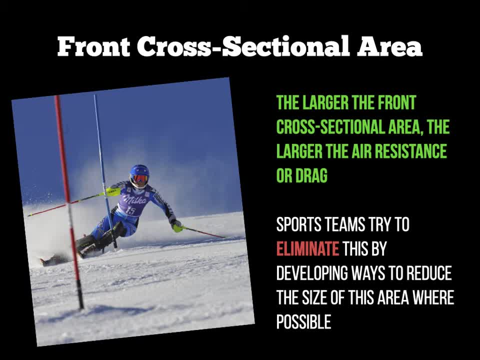 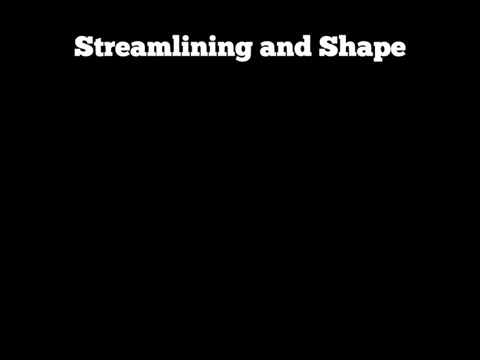 The more of the body you can bring out of the water, the more water will hit you, So you're trying to reduce that front cross-sectional area when you swim as well. Streamlining and shape technically are part of the same factor, but you can utilise them. 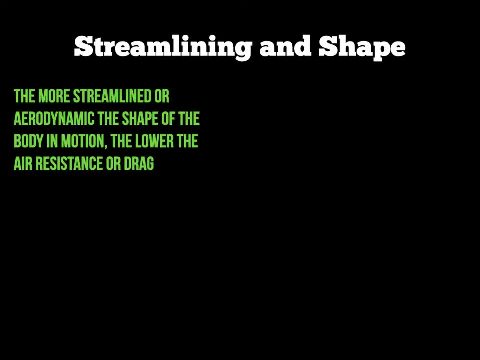 differently within exam questions. If we make an object, for example, like this: If we make an object, a body or a person more streamlined, or what we call aerodynamic, the lower the air resistance or drag through water will be. 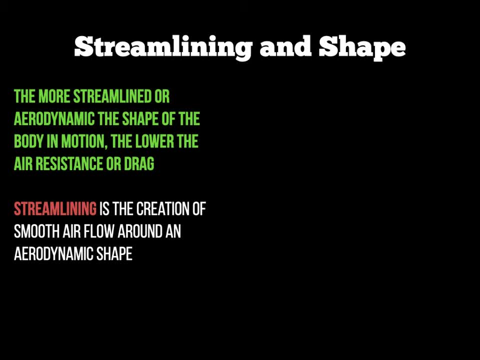 So by streamlining we mean creating a smooth airflow around an aerodynamic shape. So imagine again going back to swimming. after the diver enters the water from a dive and they go into that really tall stretch Stretched out position, They try to streamline themselves so they can minimise the pressure. 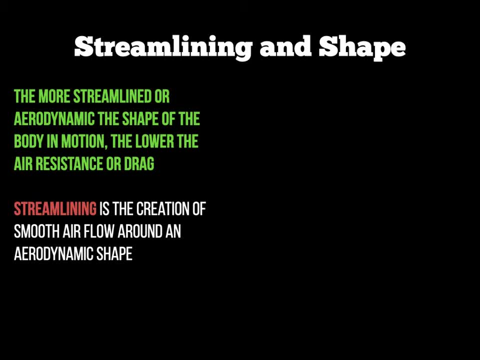 of the water against themselves so they can move faster through that water. So streamlining that position Again, think about the cyclist we spoke about in the last factor: They lower their body position, They're streamlining. Or a 100-metre sprinter: They're streamlining, They're going. 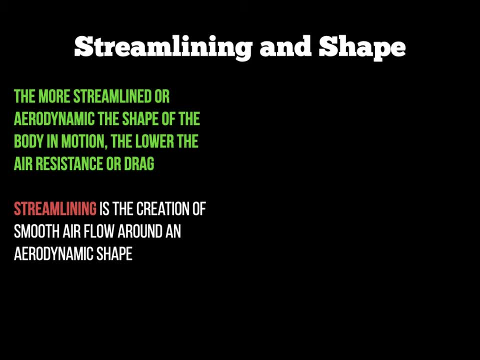 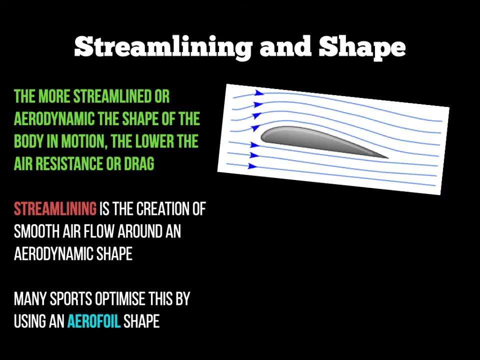 low at the start in order to minimise air resistance to accelerate. We often talk at this point of aerodynamic, Aerodynamic shapes, And the one we often talk about is an aerofoil shape, which is the picture you see on the screen. This is the common shape that will aim to reduce air. 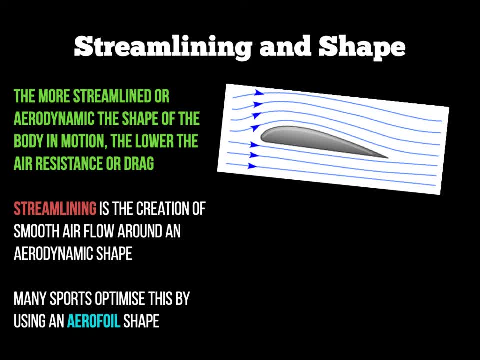 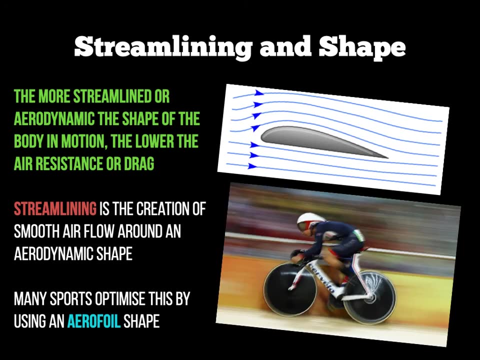 resistance and increase speed through air, which you'll meet later in the year through the concept of the Bernoulli Principle. But for this screencast, that is the shape we mean by an aerofoil shape And it's commonly seen on a cyclist's helmet. It's classic. 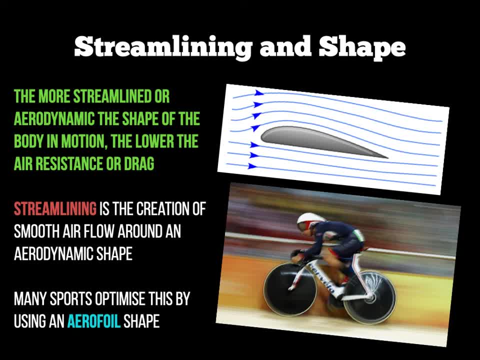 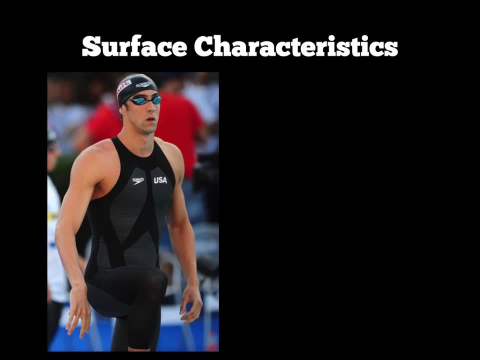 aerofoil shape And that shape will minimise the air resistance and drag for that cyclist and therefore make them go faster, accelerate through a race. The final factor is surface characteristics And logically, if we make a surface of an object that we want to push against air resistance smoother, then we can reduce that air resistance. We'll get to that in a few minutes, but we're not going to be doing that, And this is going to be the whole purpose of this video. I'm not going to be doing it at all. Instead, we're going to be giving you a little bit of information about the aerodynamic Across Air.